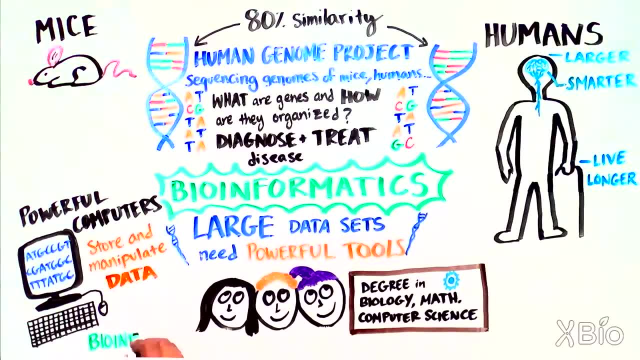 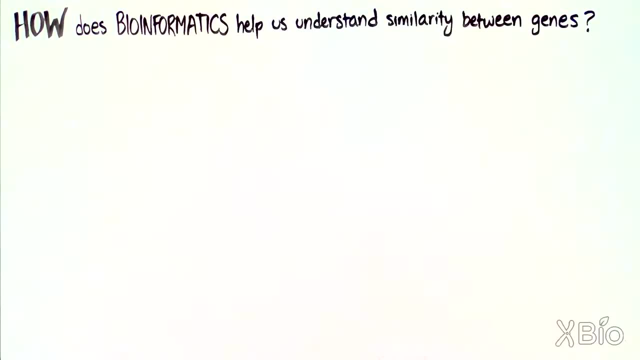 as well as math or computer science. These multidisciplinary researchers develop methods and software tools to program computers to dig through and make sense of all of this data. So how did bioinformatics help us learn that humans and mice have 80% similarity? 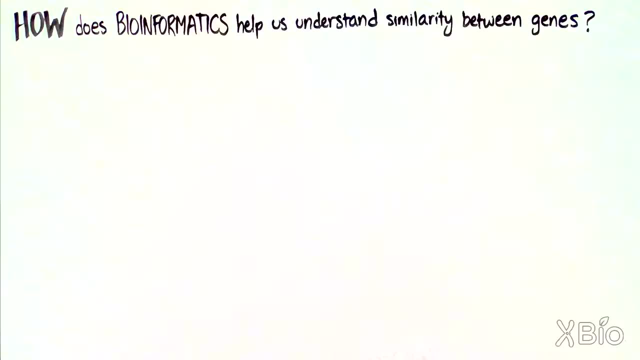 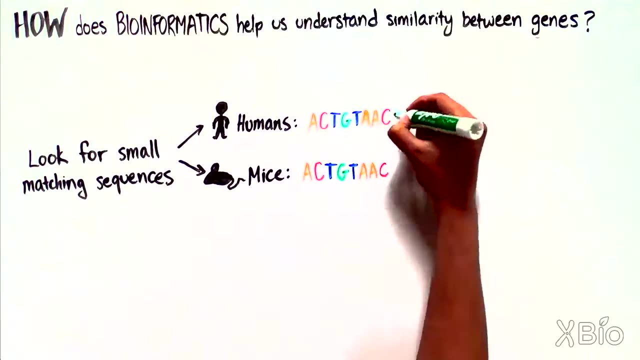 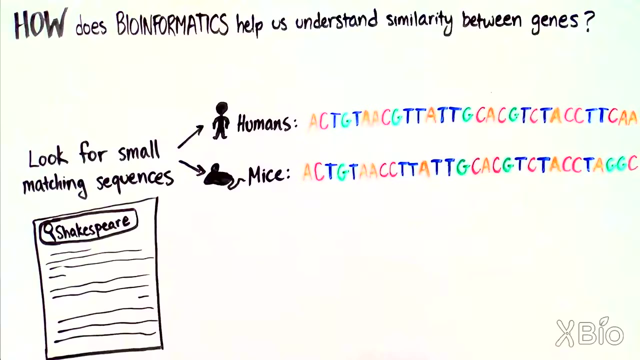 One way bioinformaticians approach this type of question is by looking for small sequences in one genome that match the other genome. This is like doing a word search on your computer, But instead of searching for the word Shakespeare in your English term paper, you scan for ATTGCACGTCTA. 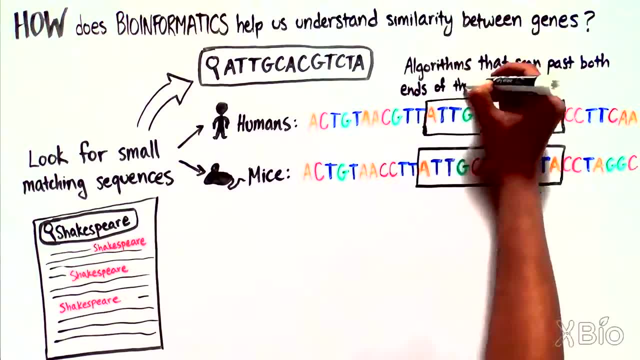 Once matching areas are found, researchers design algorithms that can scan past the ends of both sequences To see just how far the matching regions extend. So in this case, do the letters after the CTA continue to match between the mouse and human sequences? 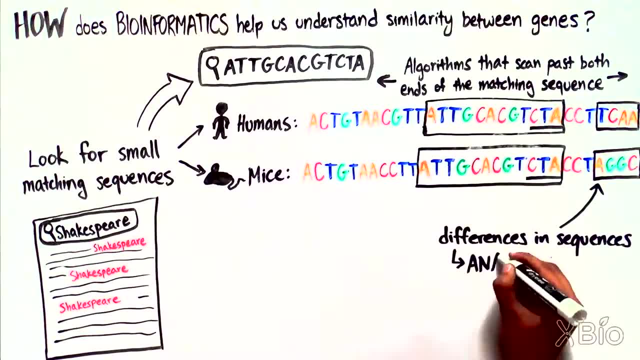 If they do not and a difference is present, we can analyze the following sequence and start to figure out which genes are involved in many of the traits that make us humans different from mice, like brain development and longevity. The flip side of this is that we can also find sequences of the genome that are more 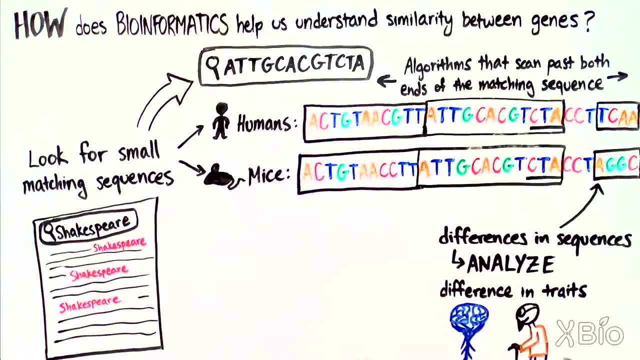 similar than the genes of other species. In addition to sharing parts of our genome with mice, humans have genes in common with plants, flies and even microscopic bacteria. These regions are called conserved genes and because they are shared across many species. 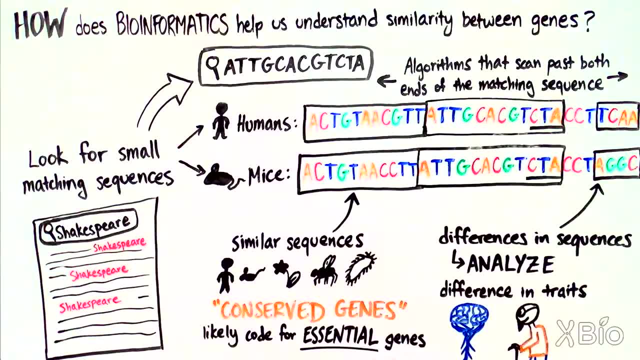 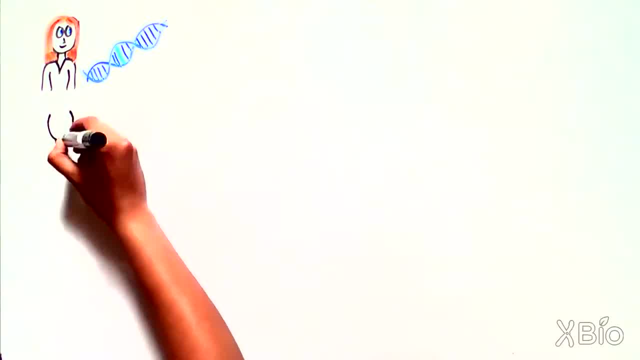 they likely code for proteins that are essential for life on earth. In addition to finding the similarities and differences between the genomes of different organisms, Sequencing technology has also allowed us to pick up differences in DNA between different people. This has been particularly important because it helps us better understand human disease. 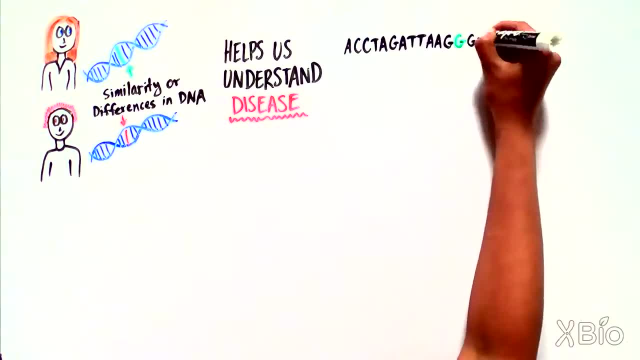 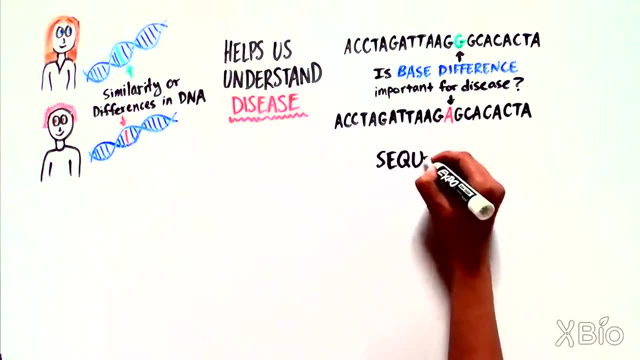 Let's say you knew a specific DNA base in a gene was different from person to person and you wanted to see if that difference was important for a disease like diabetes. You could sequence that base in 50 healthy people and 50 people with diabetes. 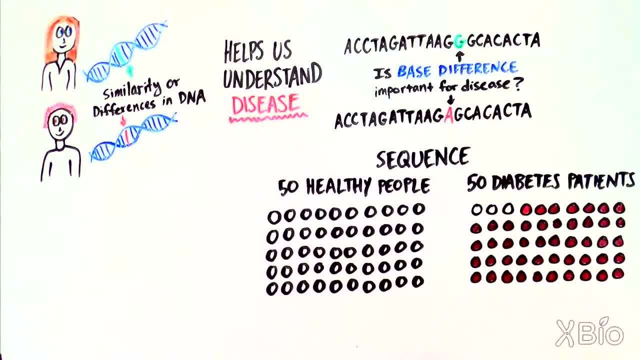 If 47 or 50 people with diabetes had an A while only 5 had a B, you could sequence that base in 50 healthy people and 50 people with diabetes. If 45 out of 50 without diabetes did, that would be strong evidence of association between.